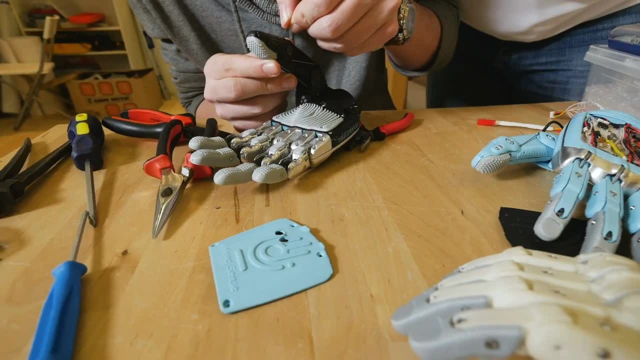 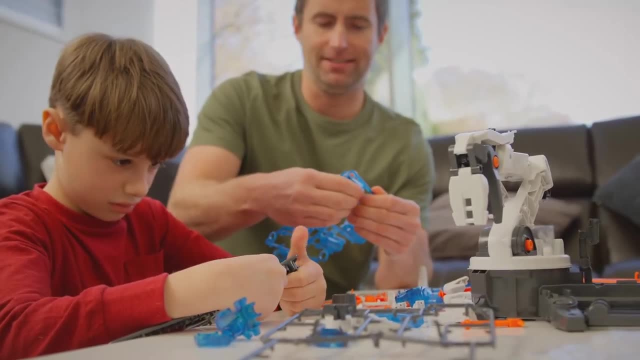 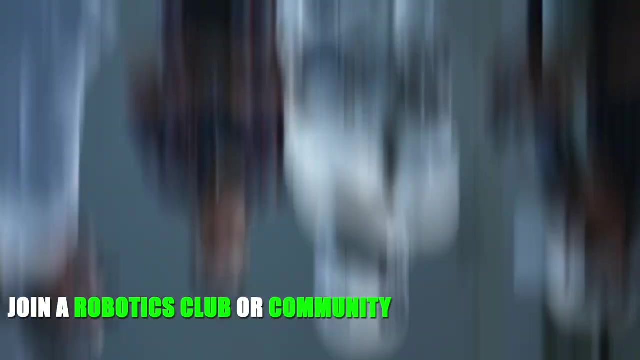 with all the necessary components and instructions to build and program a robot, so you don't have to worry about sourcing parts or figuring out how to connect everything together. Some popular robotics kits include Lego, Mindstorms, Vex Robotics and Arduino. Join a robotics club or community. Joining a. 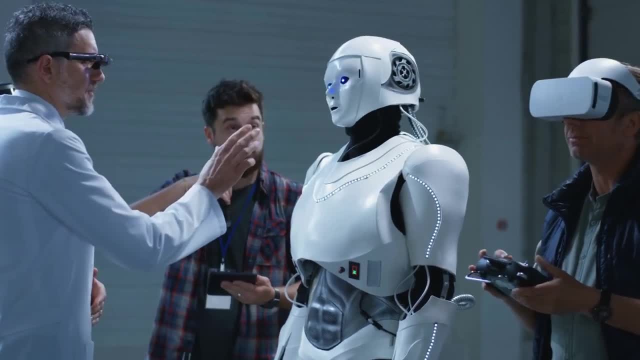 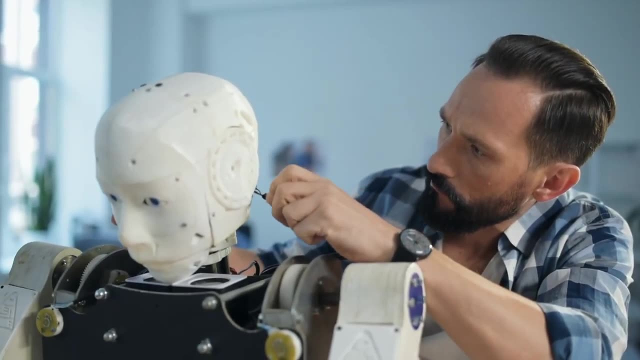 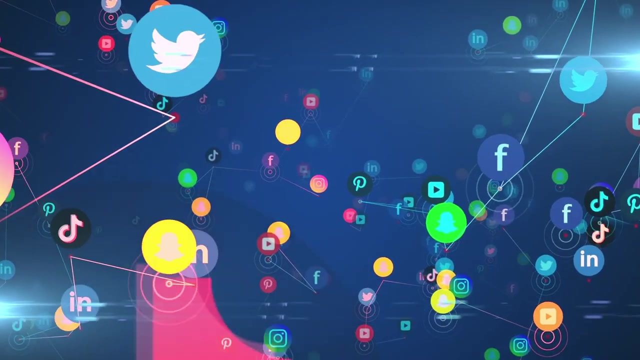 robotics club or community is a great way to connect with like-minded individuals and learn from experienced robotics engineers. Many communities offer workshops and events where you can build robots together and learn from each other's experiences. You can find robotics communities online, through social media or by attending local meetups and events. 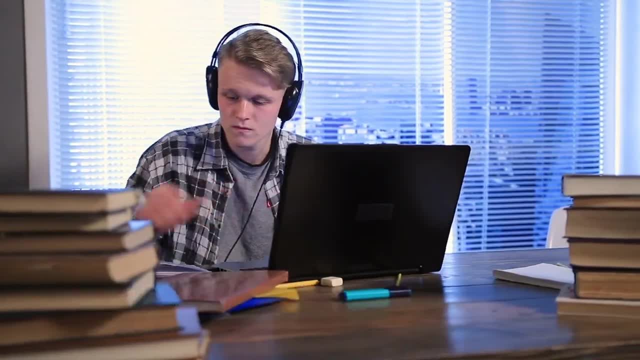 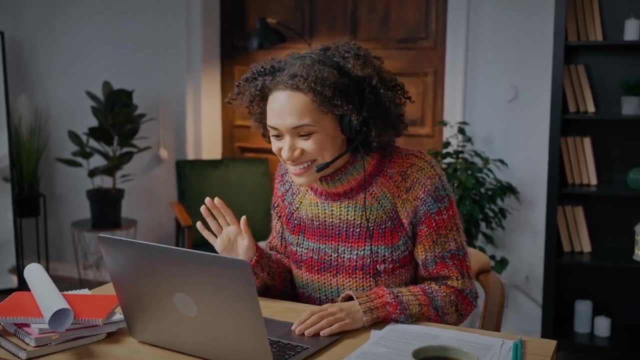 Logitech R bond today. Microsoft Office, Word, MSWordDoc, WordDocument.8. Take Online Courses or Attend Workshops. There are many online courses and workshops available to help you learn more about robotics. These courses cover a range of topics from basic electronics and programming to advanced robotics, concepts like machine learning and computer vision. 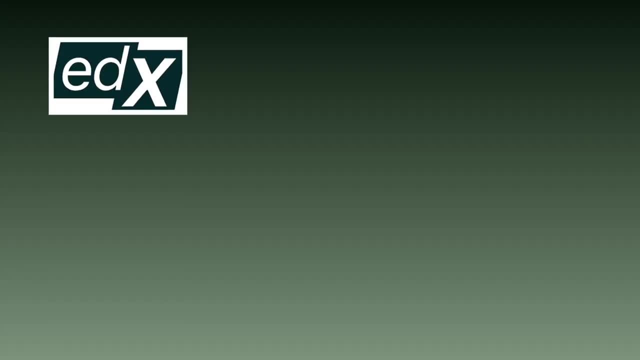 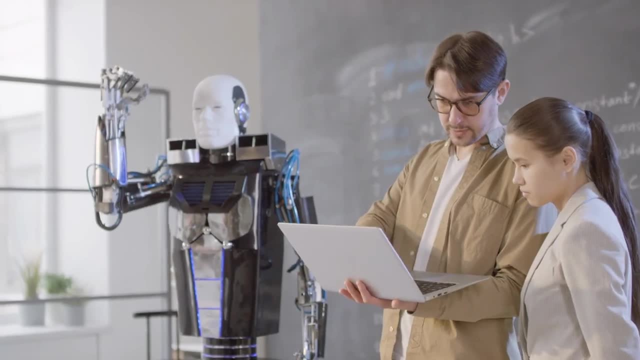 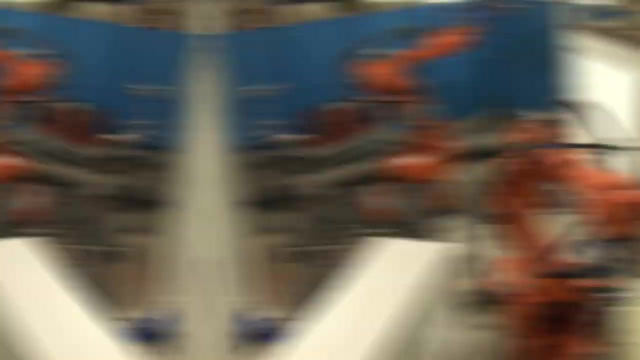 Some popular online learning platforms for robotics include EDX, Udemy and Coursera. Build Your Own Robot. Once you have a strong foundation in electronics programming and robotics, it's time to start building your own robots. There are many different types of robots you can build, from simple line-following robots to complex humanoid robots. 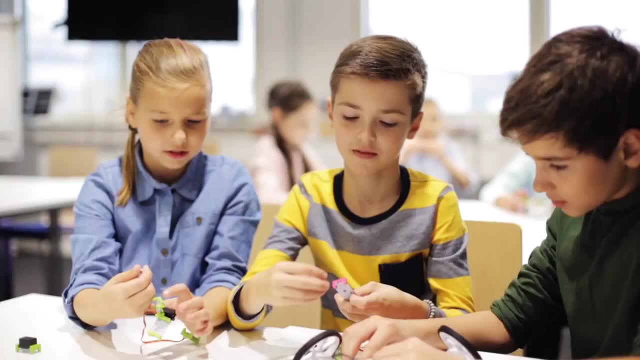 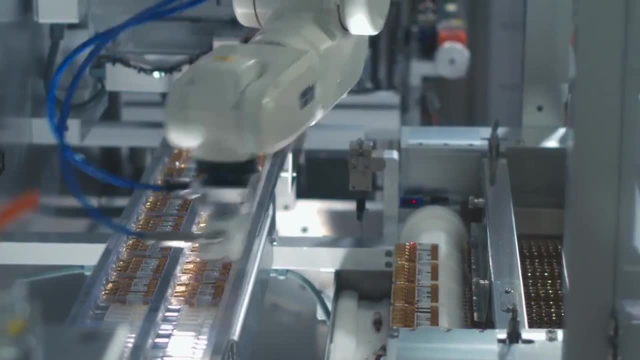 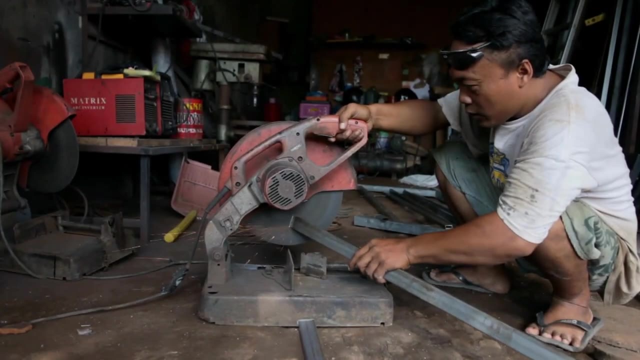 As you build more robots, you'll gain valuable experience and develop your skills as a robotics engineer. Continue Learning and Experimenting. Robotics is a rapidly evolving field, so it's important to continue learning and experimenting with your own robots, Learn about new technologies and techniques, attend conferences and workshops, read up on the latest research and developments and keep building new robots to stay at the forefront of the field. 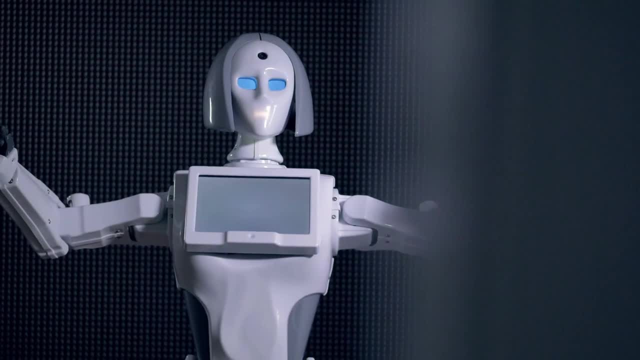 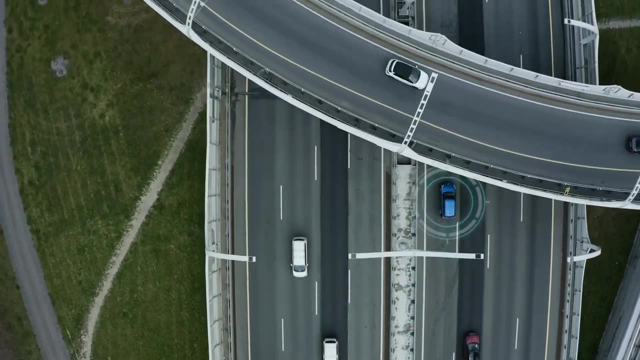 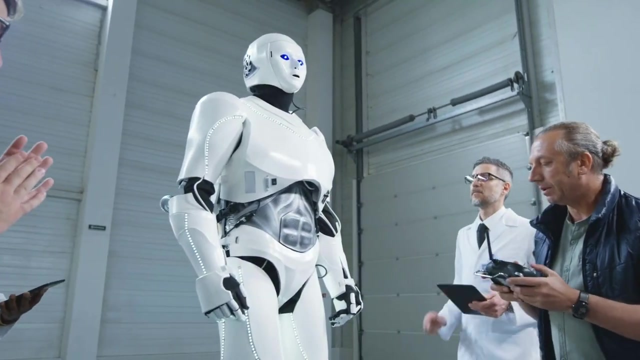 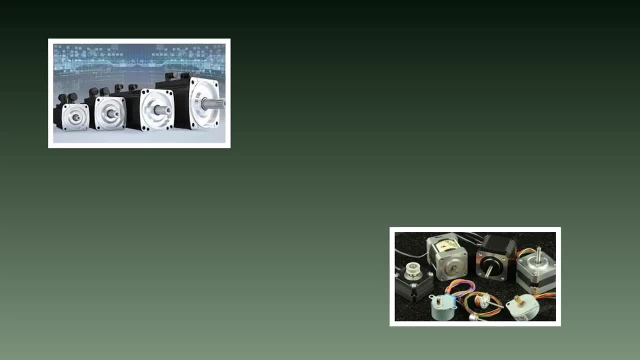 Sensors allow the robot to detect its environment and react accordingly, while actuators are used to control the movement and actions of the robot. infrared sensors, servo motors and stepper motors. Experiment with different robot designs. There are many different types of robots that you can build. 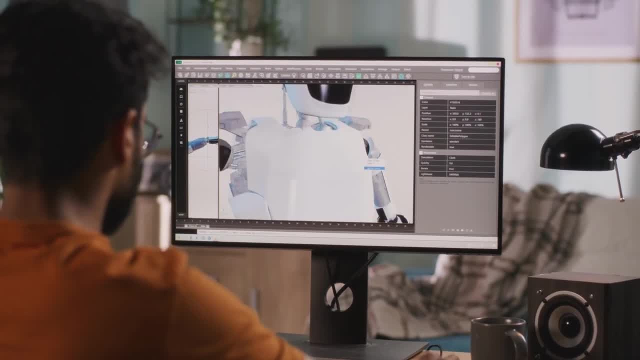 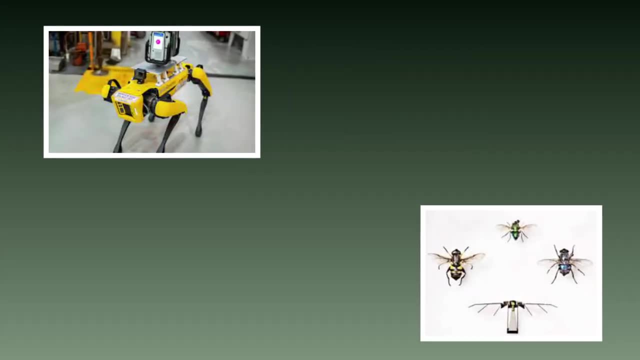 each with their own unique capabilities and design requirements. Try building robots with different designs, such as wheeled robots, legged robots or even flying robots. This will help you gain a deeper understanding of the different design principles and trade-offs involved in building robots. 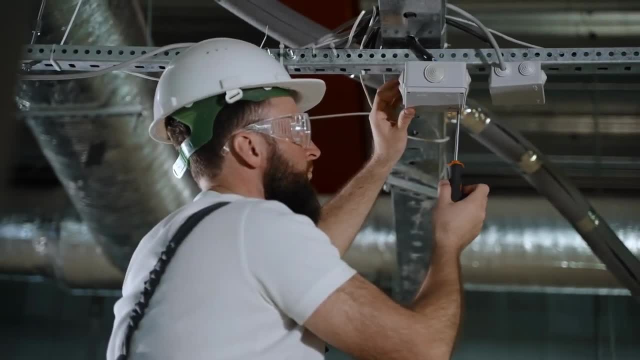 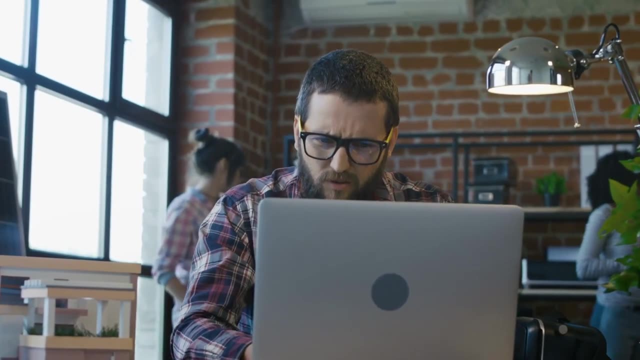 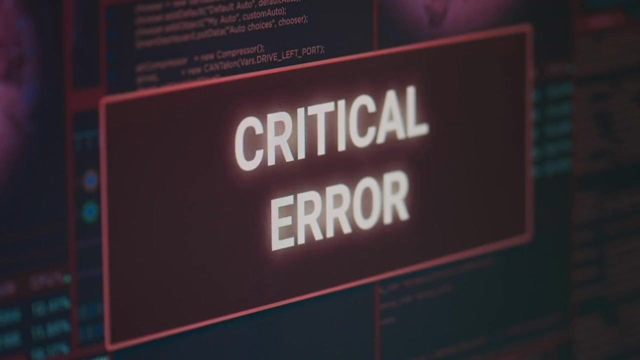 Practice troubleshooting and debugging. Building robots can be a challenging process and it's common to run into errors and problems along the way. Learning how to troubleshoot and debug your robots is an important skill for any robotics engineer. Practice diagnosing and fixing errors in your code and hardware. 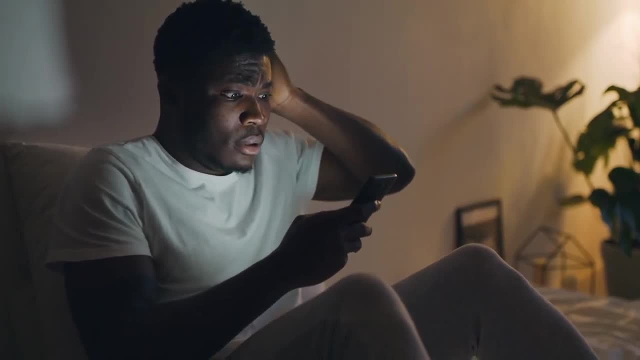 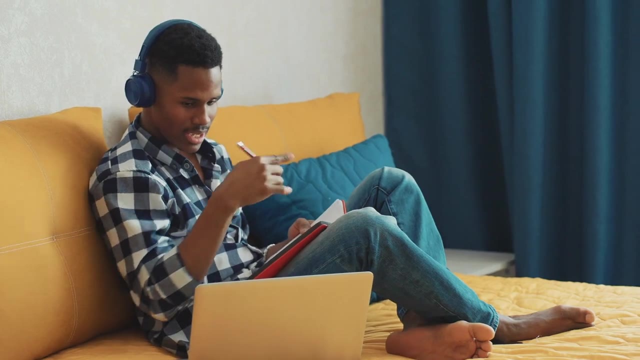 and don't be afraid to ask for help from the robotics community if you're stuck. Explore advanced topics in robotics. As you become more experienced in robotics, you may want to explore more advanced topics such as machine learning, computer vision and robotics simulation. 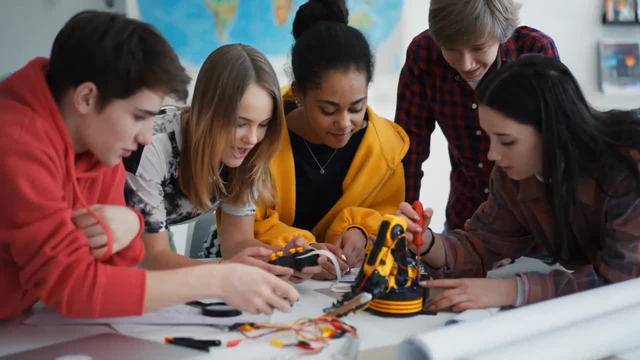 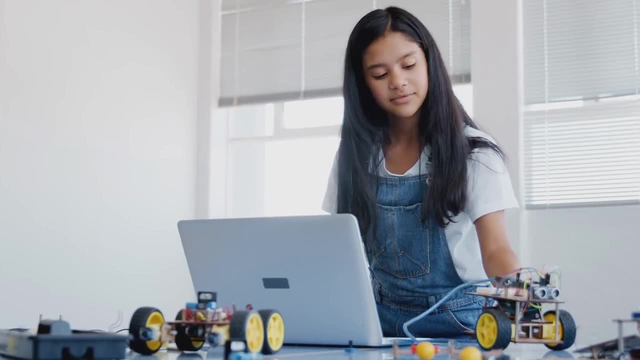 These topics can help you create more intelligent and capable robots and open up new opportunities for research and innovation in the field. There are many resources available online to help you learn these advanced topics, including online courses and research papers. Join a robotics competition. 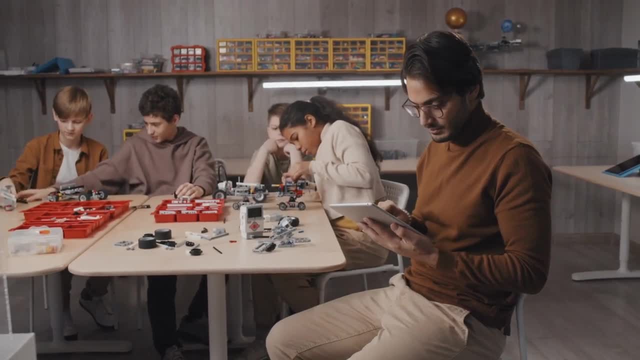 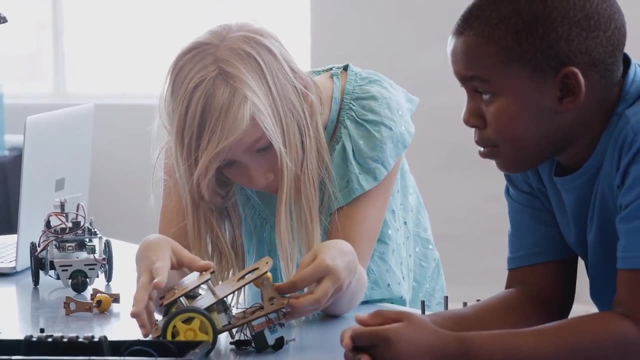 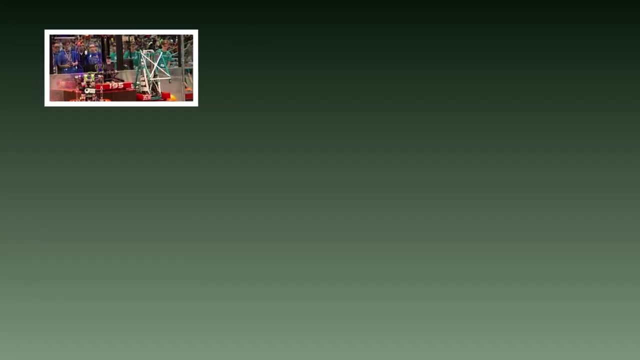 Robotics competitions are a great way to showcase your skills and compete against other robotics enthusiasts. There are many different robotics competitions available, ranging from small local events to international competitions with large cash prizes. Some popular robotics competitions include the FIRST Robotics Competition, RoboCup and the DARPA Robotics Challenge. 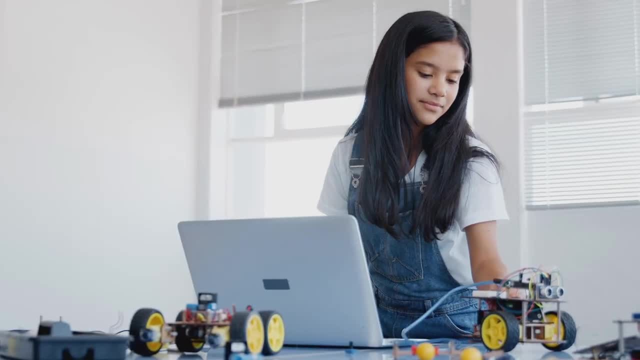 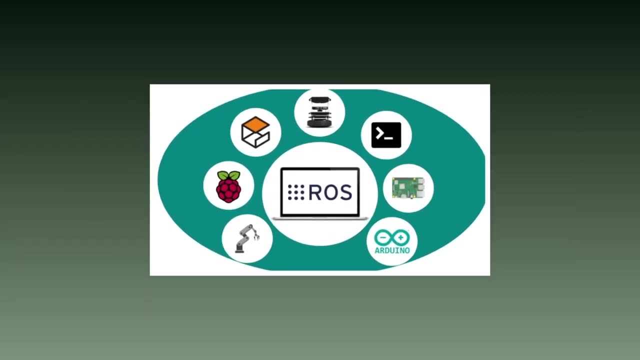 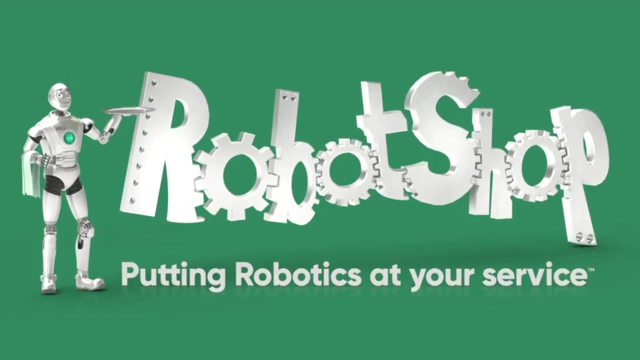 In addition to the tips above, there are many resources available to help you get started in robotics. Some popular robotics resources include ROS Robot Operating System, a popular open-source software framework for building robots. Robot Shop, an online retailer that sells a wide range of robotics components and kits. 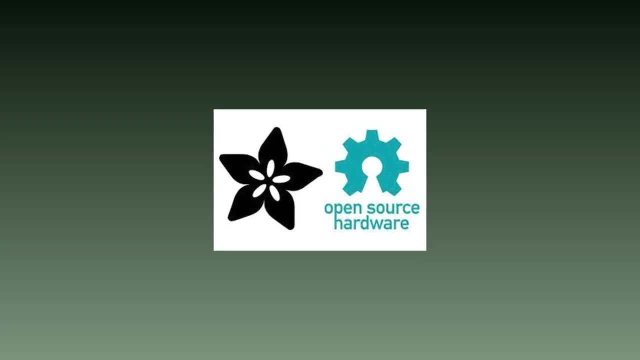 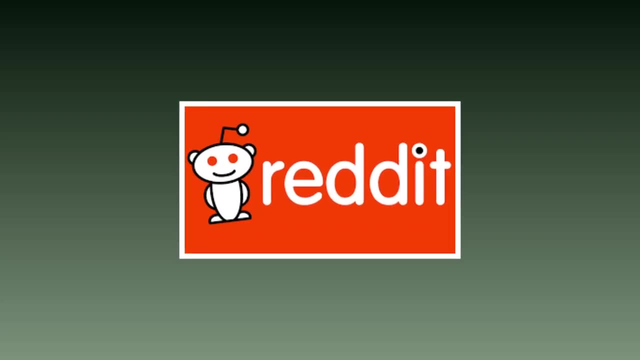 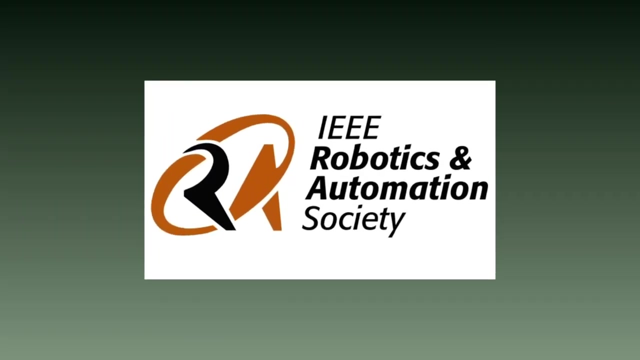 Adafruit, an online retailer that specializes in electronics components and DIY electronics projects. Reddit, the robotics subreddit, is a great place to connect with other robotics enthusiasts and learn about the latest developments in the field. IEEE Robotics and Automation Society, a professional organization dedicated to advancing the field of robotics and automation. 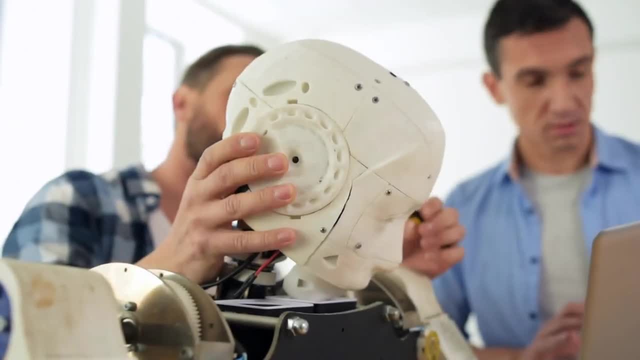 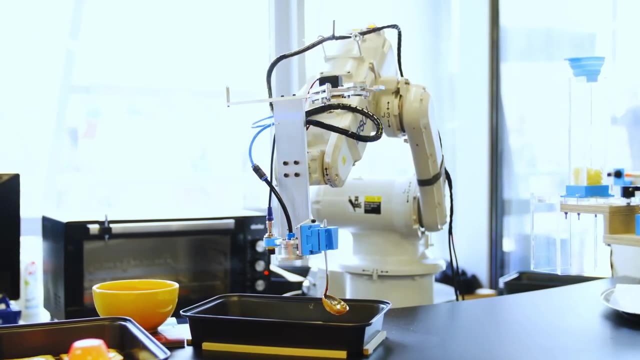 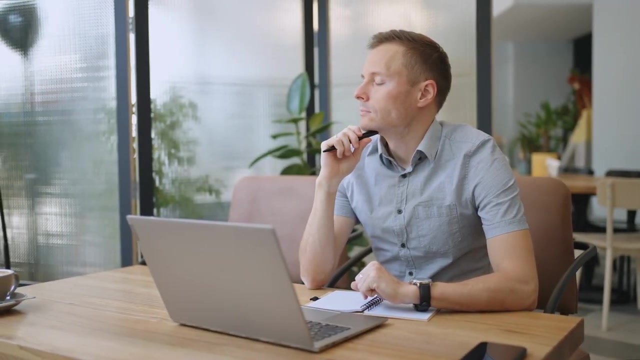 Network with other robotics enthusiasts. Networking with other robotics enthusiasts can provide you with valuable insights and feedback, as well as help you stay up-to-date on the latest trends and developments in the field. Join online forums, attend local meetups and events, and consider participating in robotics hackathons to connect with other robotics enthusiasts. 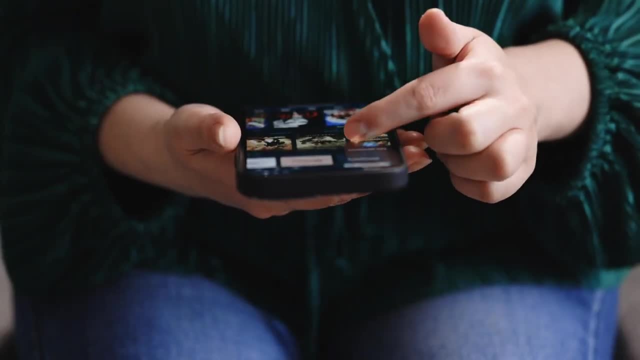 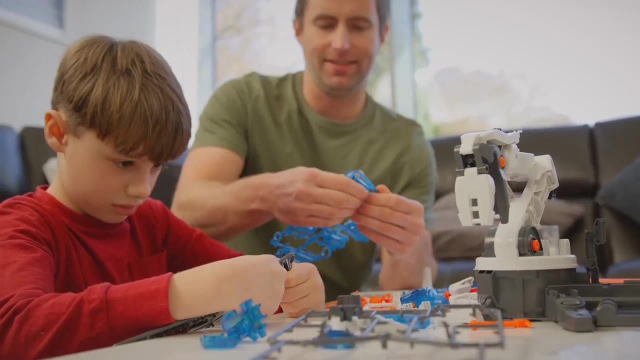 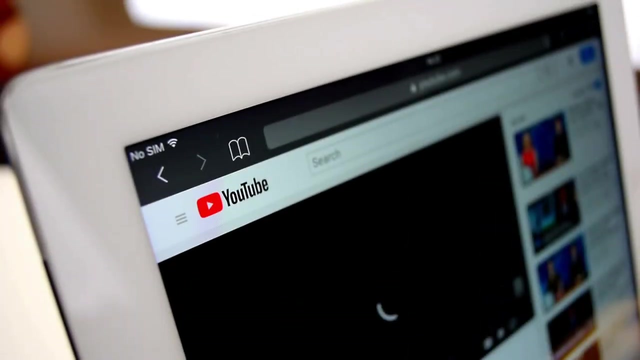 Build a portfolio of robotics projects. Building a portfolio of robotics projects can help you showcase your skills and experience to potential employers or clients. Start with simple projects and work your way up to more complex ones, documenting your progress along the way. You can also contribute to open-source robotics projects. 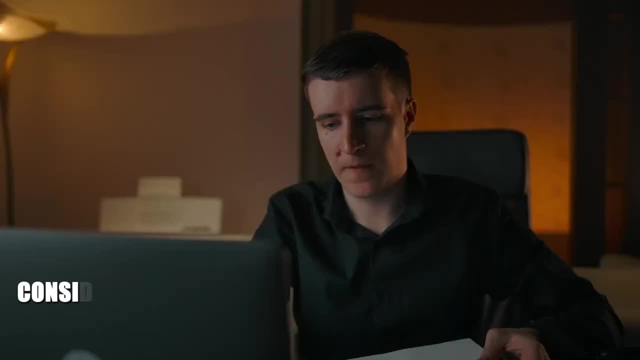 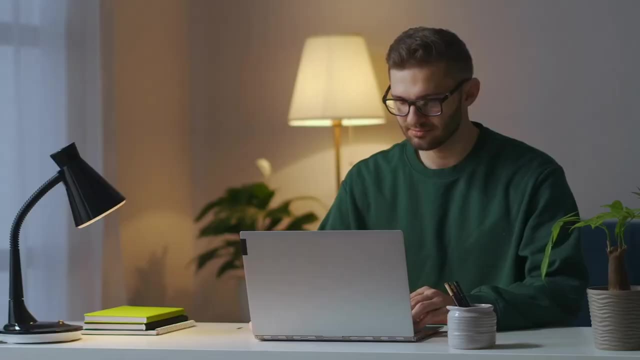 or publish your own research papers to build your portfolio. Consider pursuing formal education in robotics. While it's possible to learn robotics on your own, pursuing formal education in the field can provide you with a deeper understanding of the principles and techniques used in robotics. 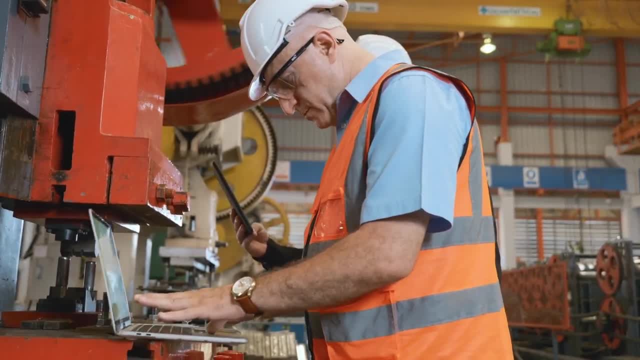 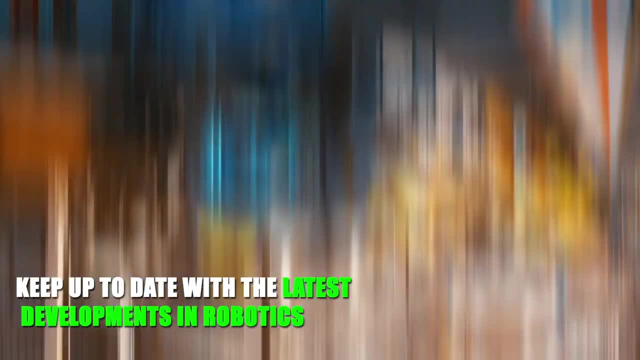 Consider enrolling in a robotics-focused degree program or taking robotics courses at a local school. Consider joining a local college or university. Keep up-to-date with the latest developments in robotics. The field of robotics is constantly evolving, with new technologies and techniques being developed all the time. 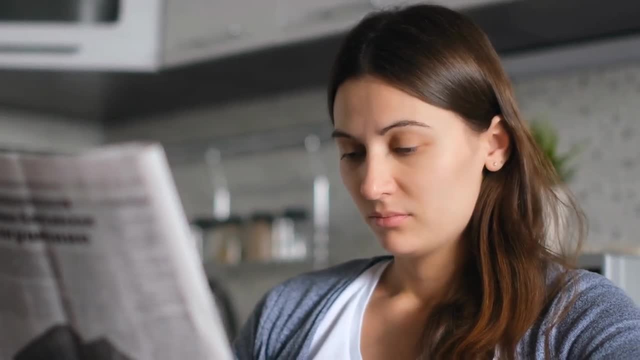 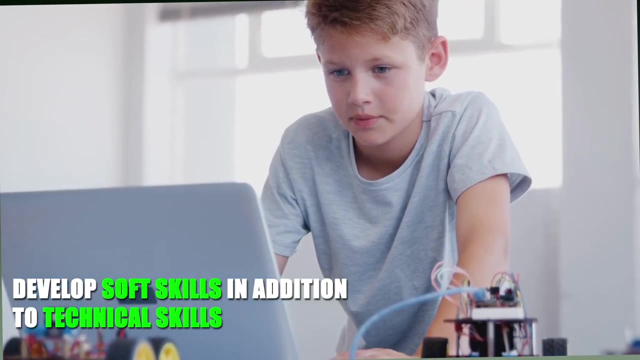 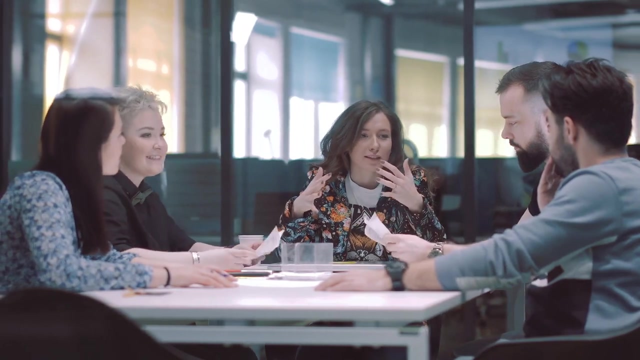 Stay up-to-date with the latest developments by reading research papers, attending conferences and following robotics news websites and blogs. Develop soft skills in addition to technical skills. In addition to technical skills, developing soft skills such as communication, teamwork and problem solving. 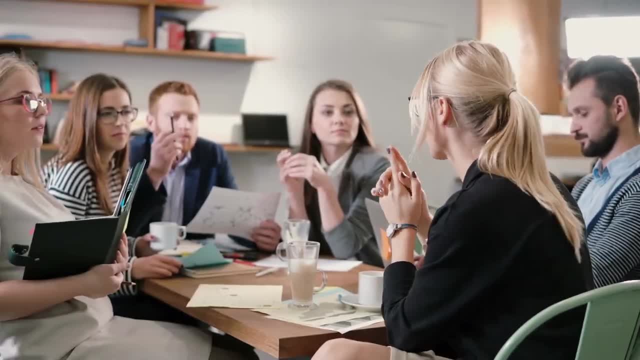 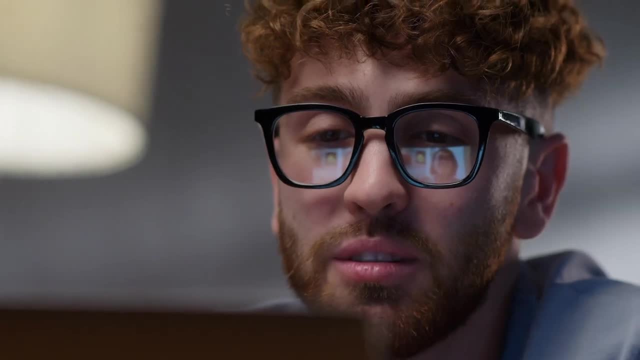 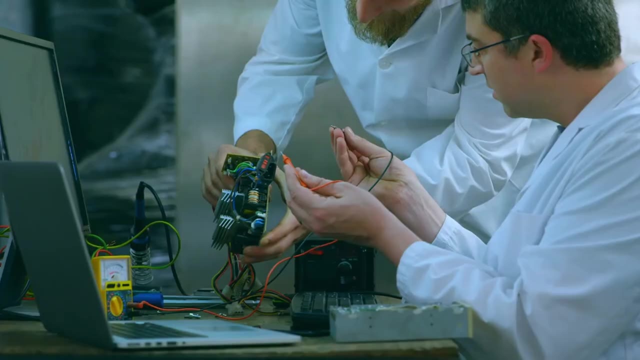 can be valuable in a robotics career. Practice working in teams and communicating effectively with others, and consider taking courses or attending workshops to develop your soft skills. Explore career opportunities in robotics. There are many different career paths available in robotics, ranging from robotics engineering and software development to research and academia. 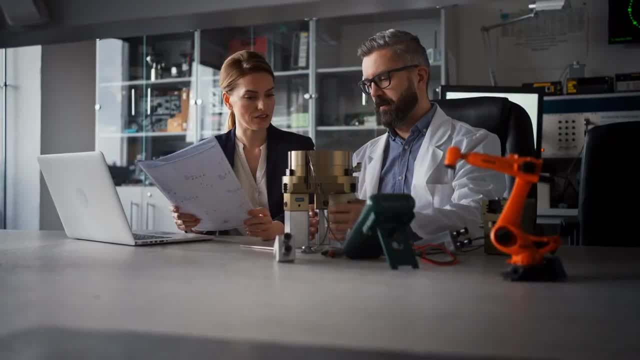 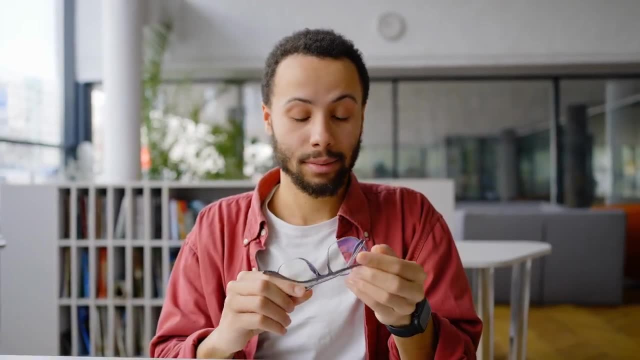 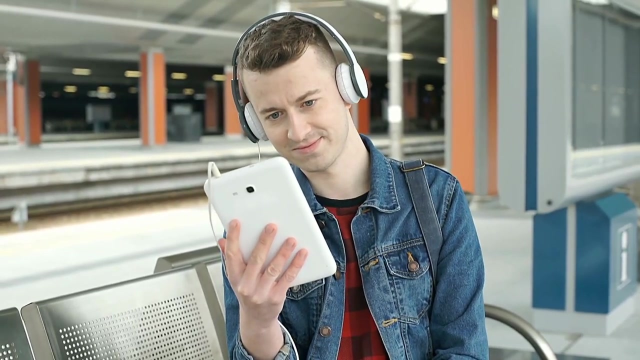 Explore different career opportunities in the field and consider what path may be the best fit for your skills and interests. By following these additional tips, you can further enhance your knowledge and skills in robotics and prepare yourself for a rewarding career in the field. If you enjoyed this video and found it helpful in getting started in robotics,